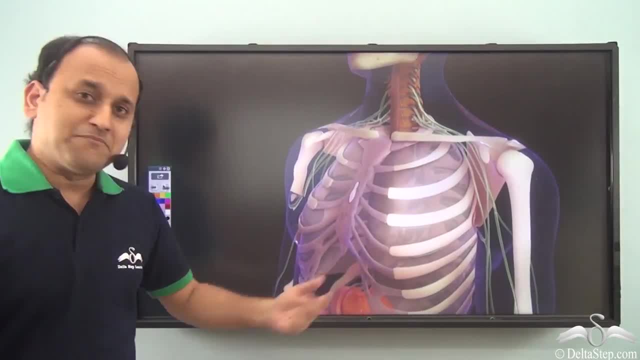 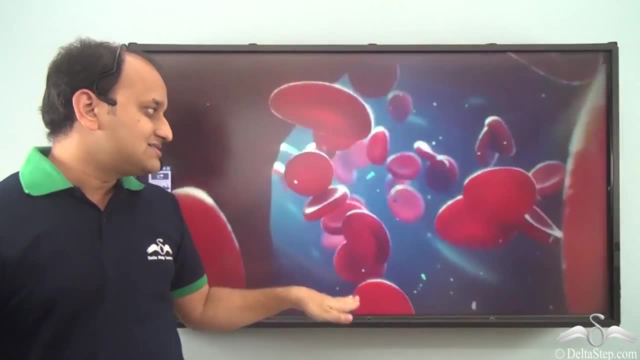 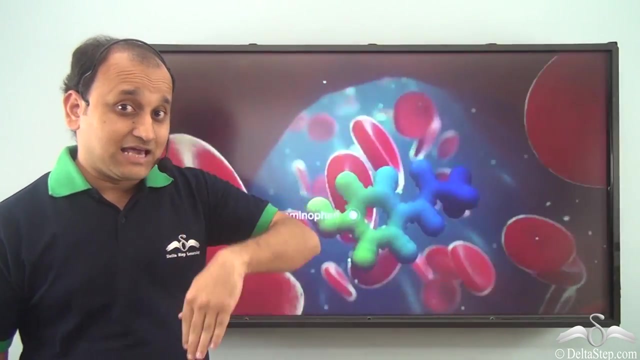 chemicals. when it is ill, Then we take medicine, isn't it? Now, what are these medicines? Well, these are chemicals. So once these chemicals are released in our body, well, these chemicals travel inside our body, and then these chemicals try to react with other chemicals. 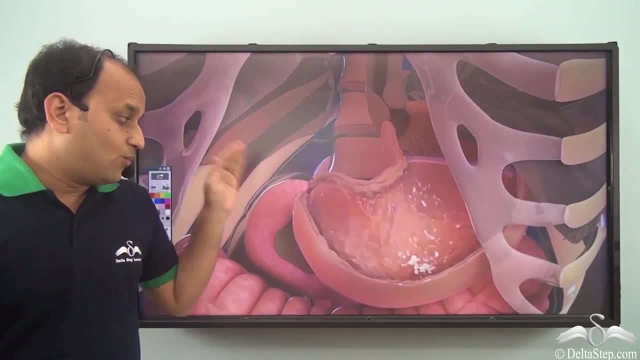 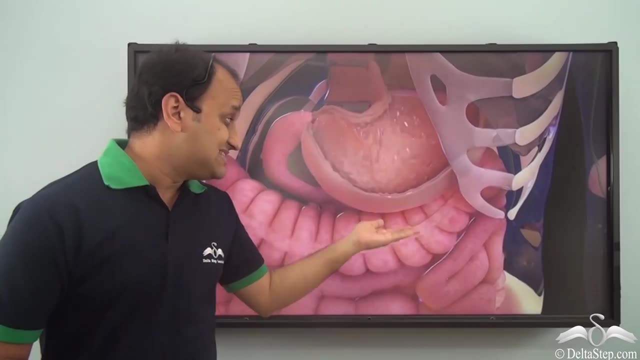 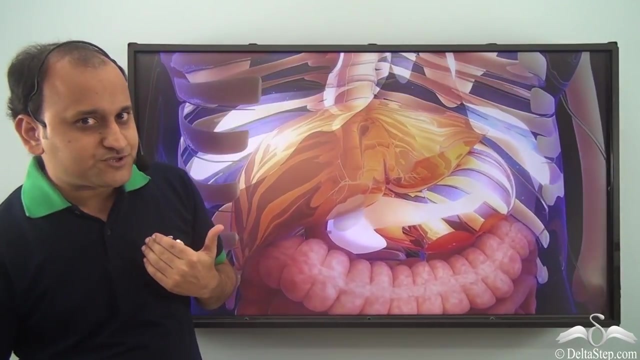 which are already present in our body. So what are these medicines? These are, again, products of chemistry, that is, they are chemicals. and once they enter our body, well, they are absorbed by different parts of the body. and after absorption, what happens? Well, all. 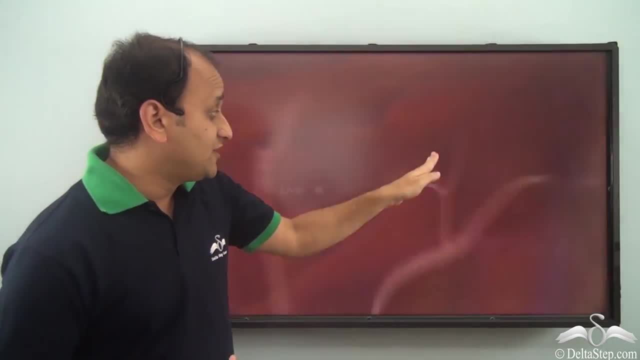 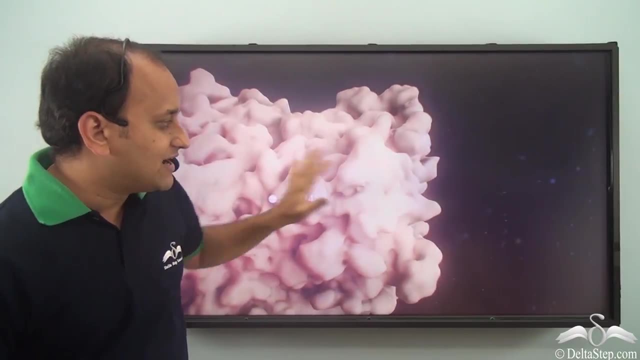 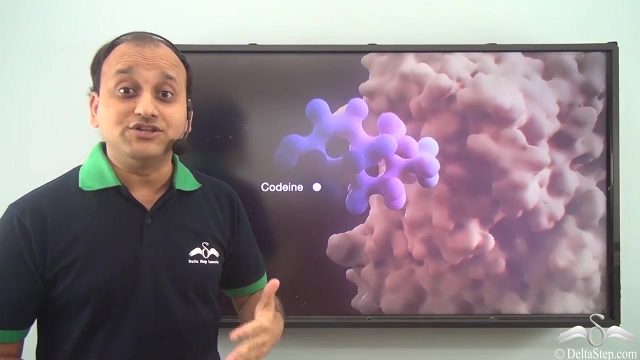 these chemicals start travelling to different organs of the body and there these chemicals are trying to react with other chemicals already inside the body and, as a result, unwanted chemicals are released which exit our body through different excretion means. So what exactly happened here? 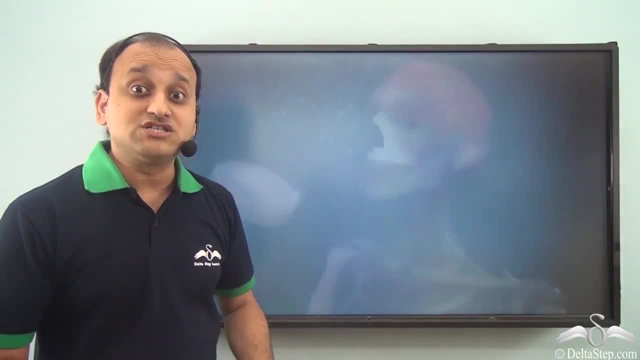 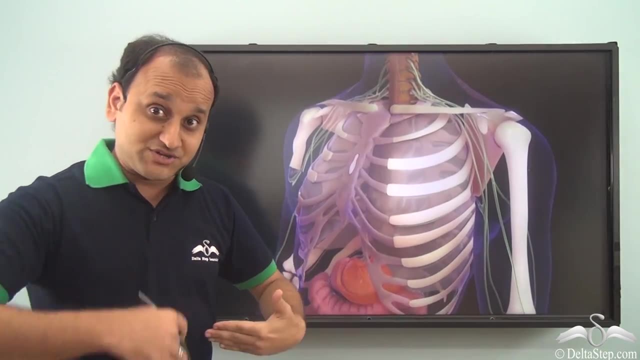 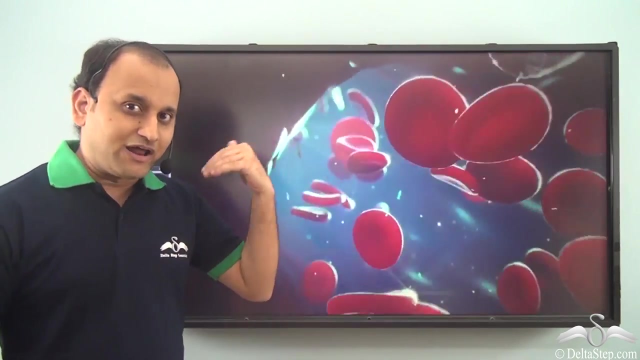 A number of chemical reactions which occurred because we took a medicine. So even a medicine is a product of chemistry and that triggers a number of chemical reactions inside our body. So when we fall ill it is chemistry that helps us to fix that particular illness. 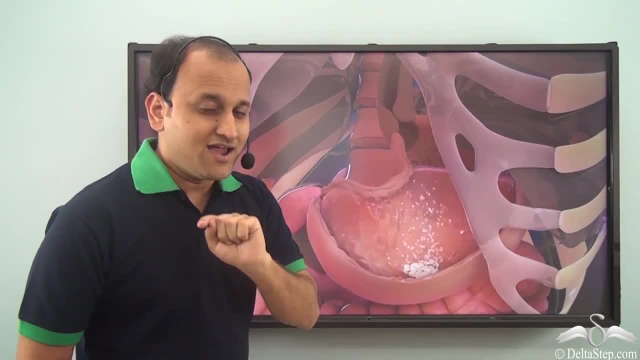 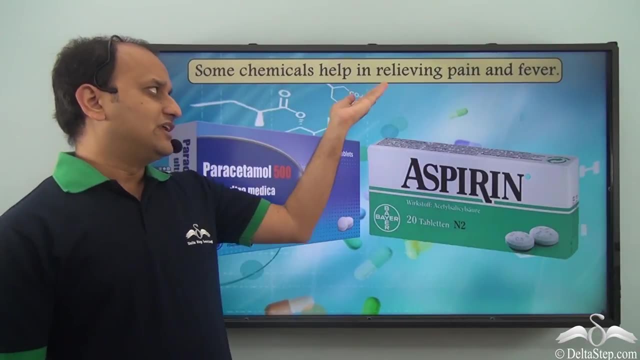 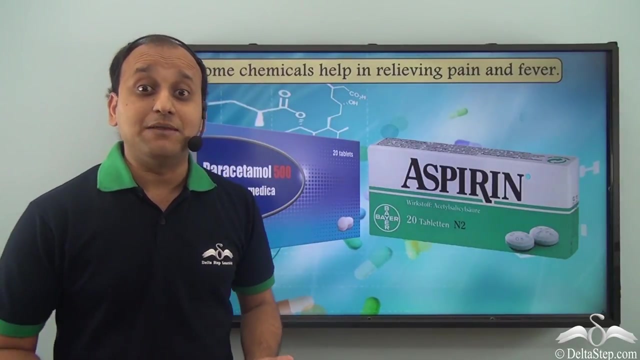 So even for staying healthy, we need chemistry. Now, what are some common chemicals that help us to relieve pain and fever? Well, Paracetamol and Aspirin are two of the medicines which help us relieve pain and fever, and these are: 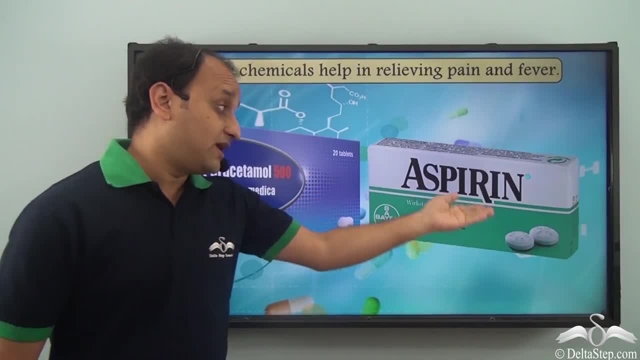 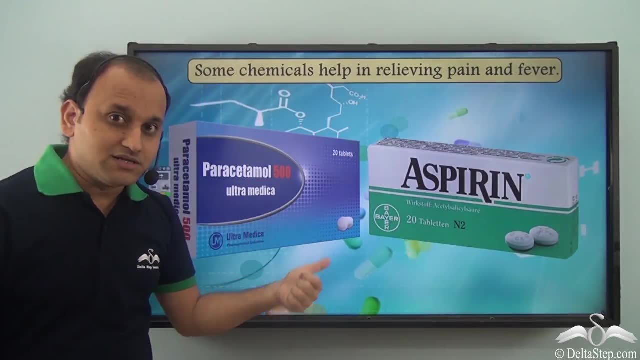 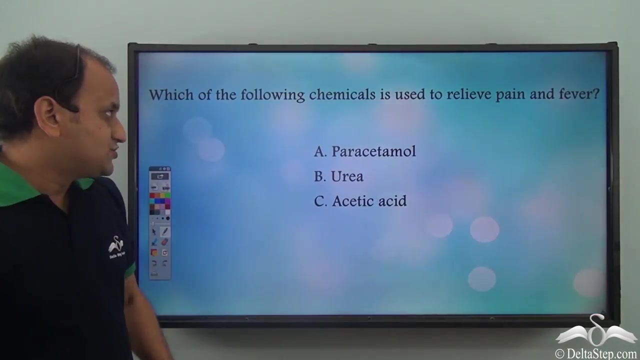 nothing but chemicals. So Paracetamol and Aspirin are names of some chemicals that help us relieve pain and fever. So without these chemicals we cannot get rid of these problems- Excuse me, problems of our body. So can you answer this? Which of the following chemicals is used to? 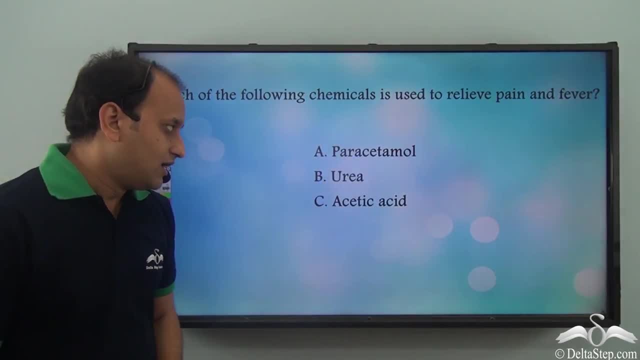 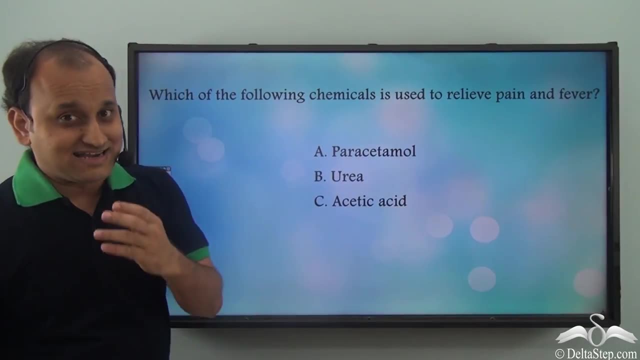 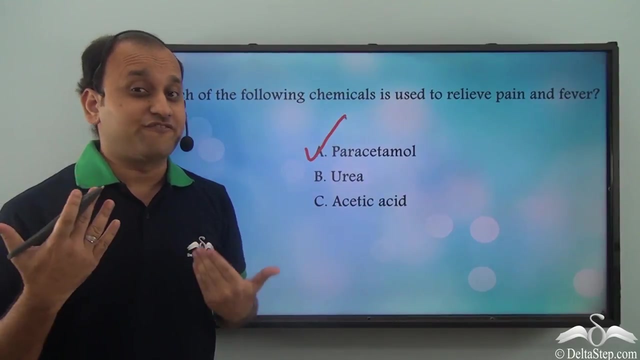 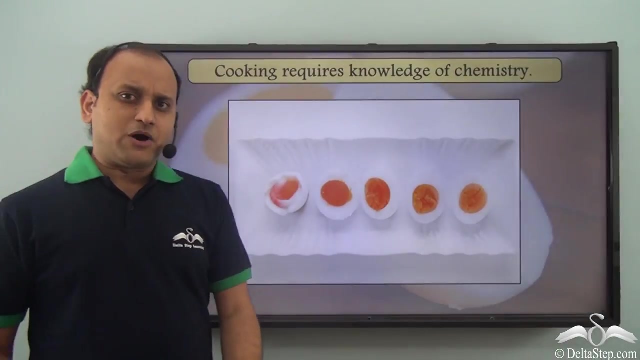 relieve pain and fever. Is it paracetamol, is it urea or is it acetic acid? What do you think? Well, the answer is paracetamol. So paracetamol is a chemical, that is a product of chemistry that helps us get rid of pain and fever. So that was about medicines. But 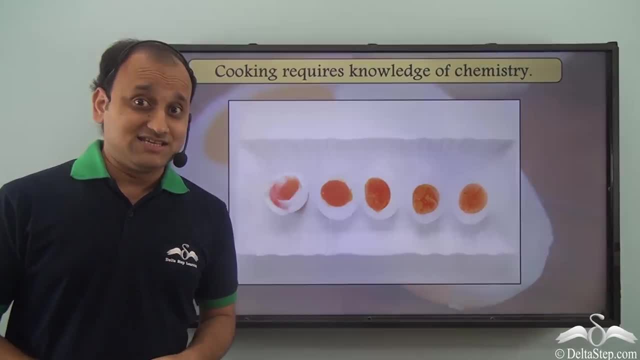 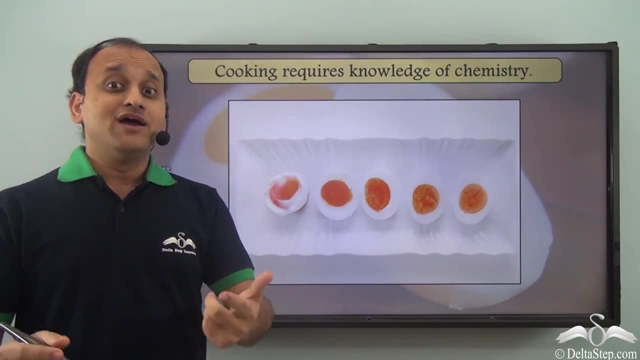 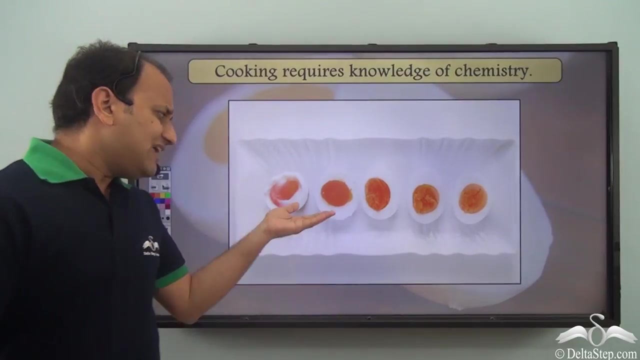 we also need to eat food to keep us healthy, isn't it? Now? even cooking food requires knowledge of chemistry. So if you want to become a chef, you need to know chemistry. Now you must be thinking how- Let's take a very common example of an egg. Now we eat. 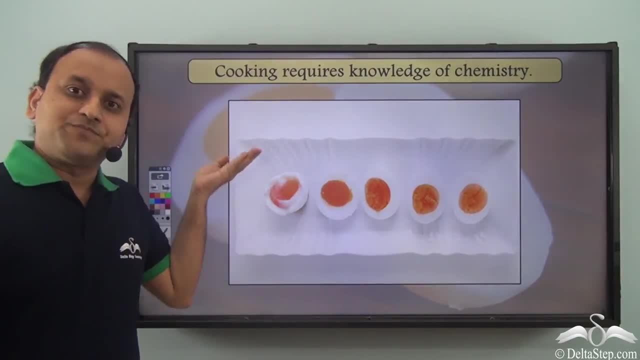 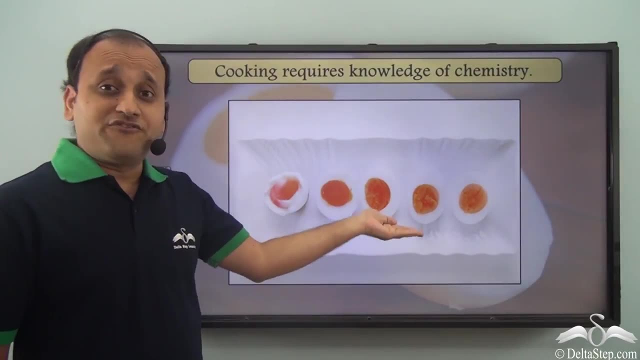 egg in different forms. Sometimes we want to eat an egg in different forms. Sometimes we want to eat an egg in different forms. Sometimes we want a runny yolk, Sometimes we want a liquid yolk, and sometimes we want a soft yolk or maybe hard yolk. So how do we achieve all these different phases of the 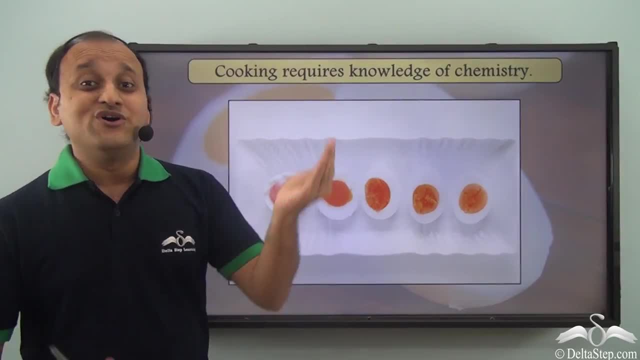 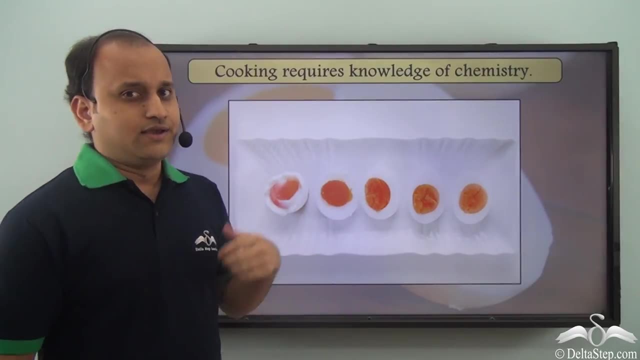 same egg. Well, for that we need to know the chemistry of egg. So, as you can see, egg has two major parts: the yolk and the egg white. Now, whoever is a chef, he knows the chemistry of both these components. 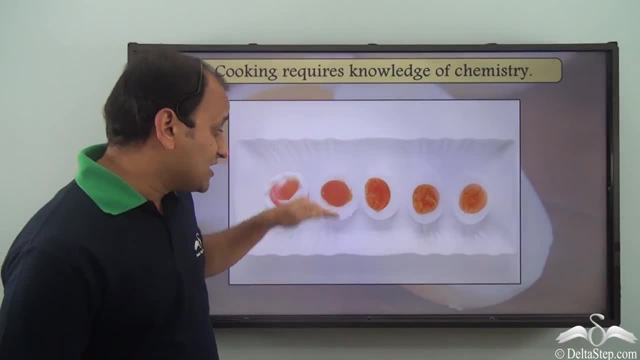 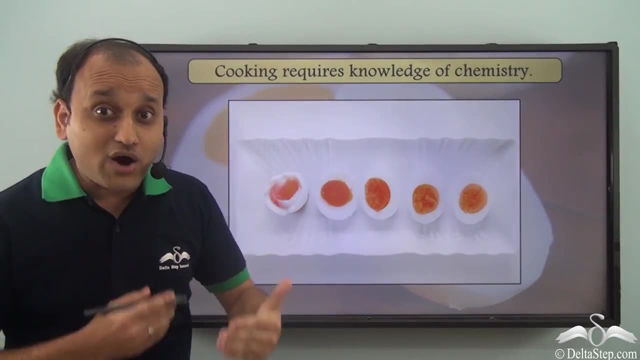 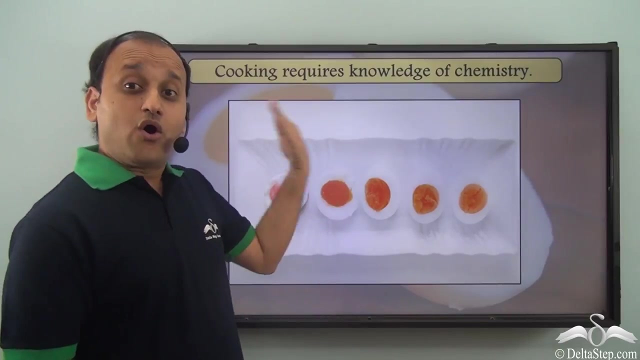 So a chef knows how much the white part needs to be cooked, how much the yolk part needs to be cooked, And accordingly a chef can adjust the temperatures or the time of cooking so that only one or both parts are cooked properly. So all this is possible only when 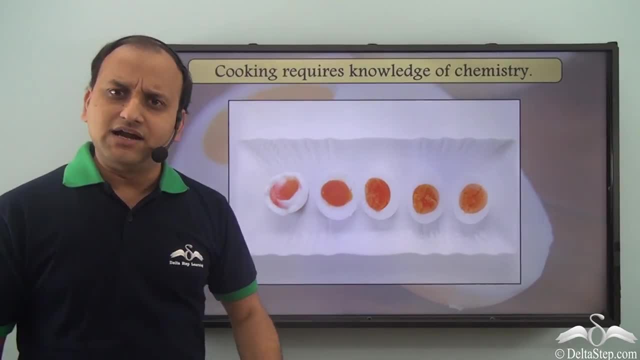 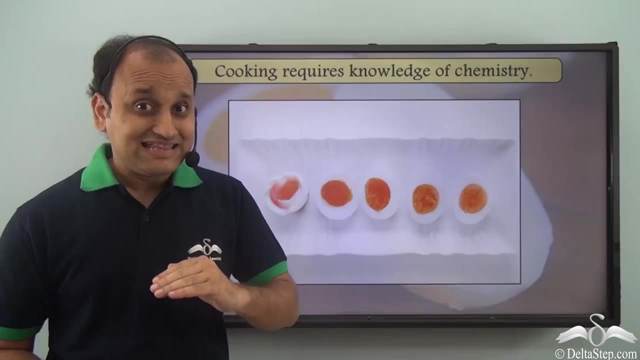 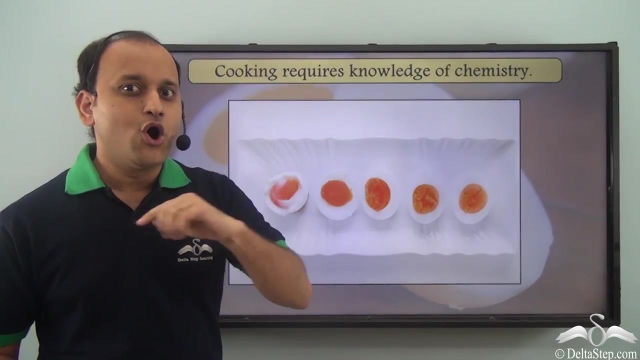 we know the chemistry of this food. Similarly, while cooking any particular item, you need to know the chemistry of that particular item. Only then you will be able to cook it in the right proportion. So if you want to become a chef, you need to know chemistry. 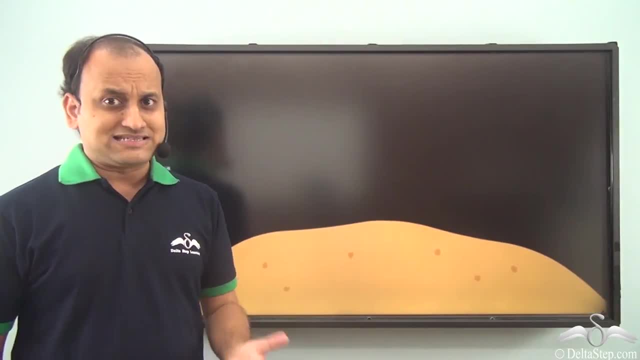 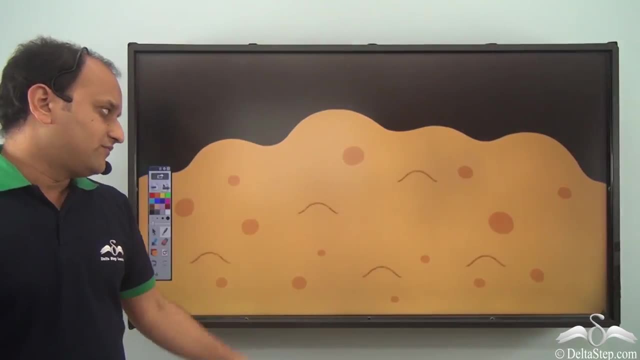 Let's take an example of a cookie. So something as simple as a cookie requires huge knowledge of chemistry. So what do you see here? Well, we see different reactions which happen inside a cookie Before we knew about the chemical reactions. so we know about the chemical reactions. 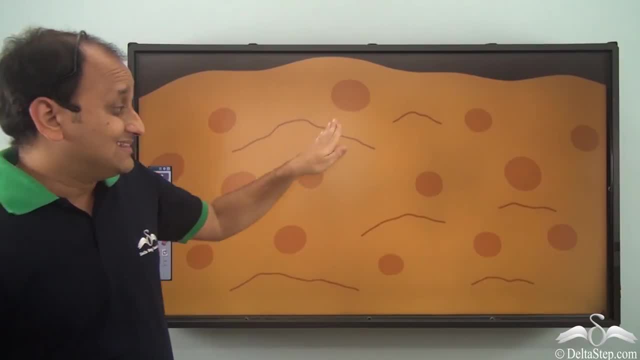 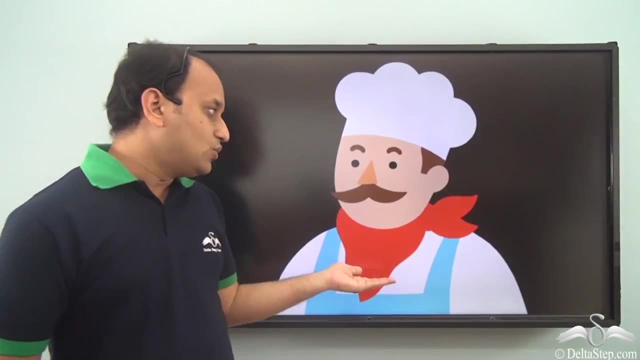 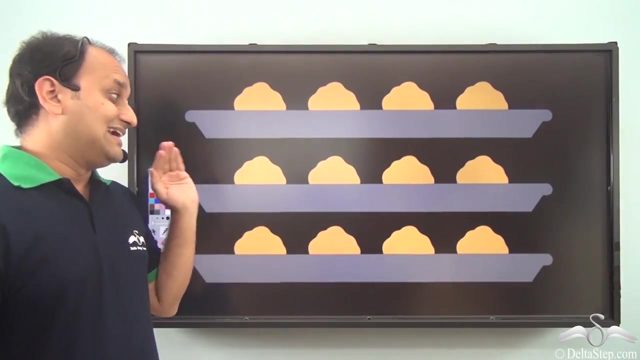 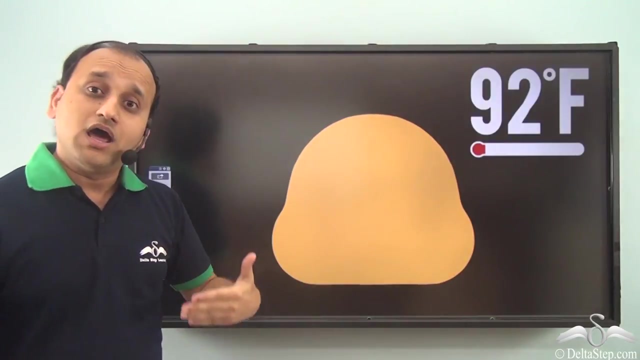 you get to eat it. So, while cooking, this particular cookie undergoes a number of chemical changes. and how do these chemical changes take place? Well, the chef, who is actually a chemical scientist, decides when to cook and how to cook the cookie. So, inside a cookie, there are a number of ingredients, and every 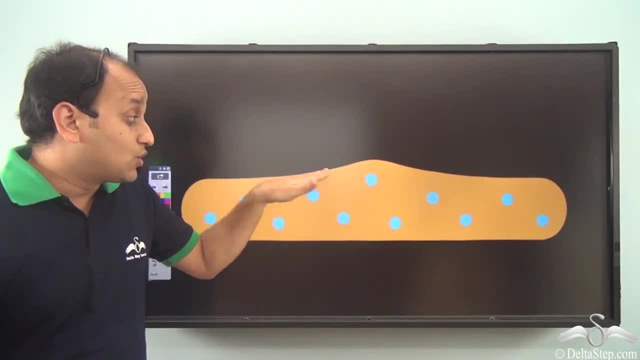 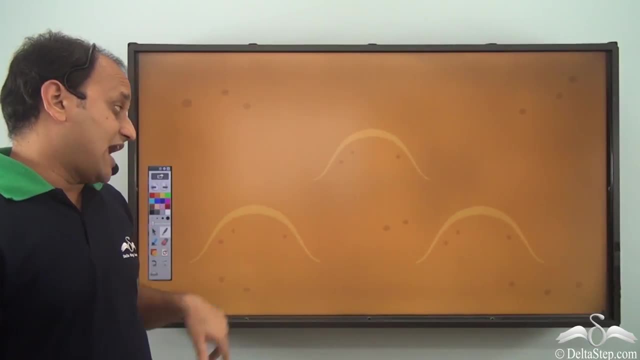 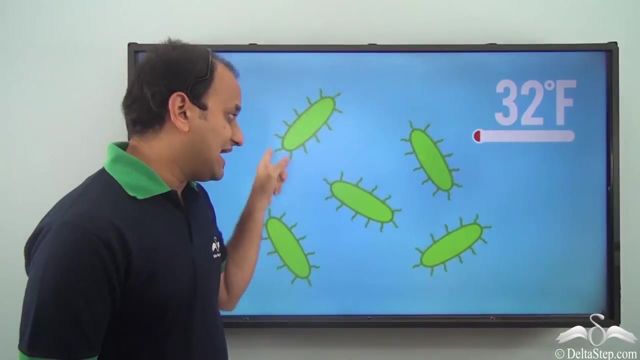 ingredient behaves differently when cooked at different temperatures and, as you can see, with changing temperatures there are changing chemical reactions and also there are different germs which, if eaten, can make you ill. Now, how do you take care of all these germs? Well, there is a particular temperature to which 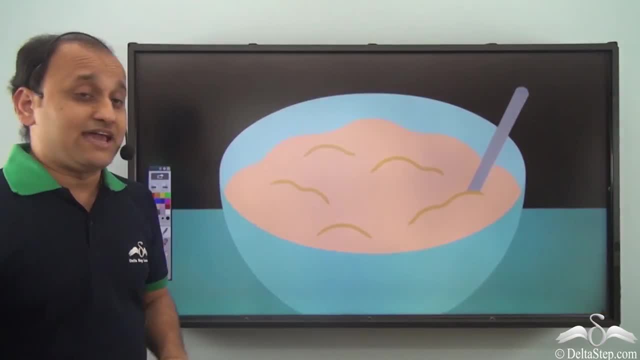 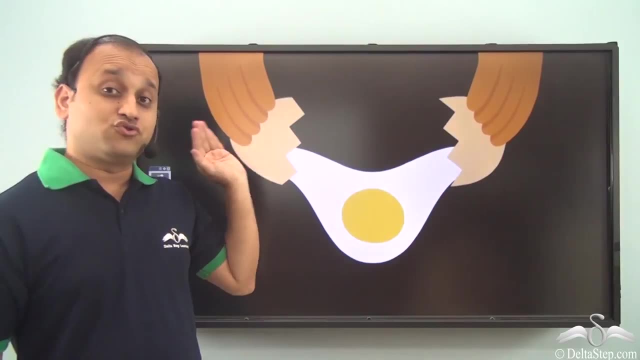 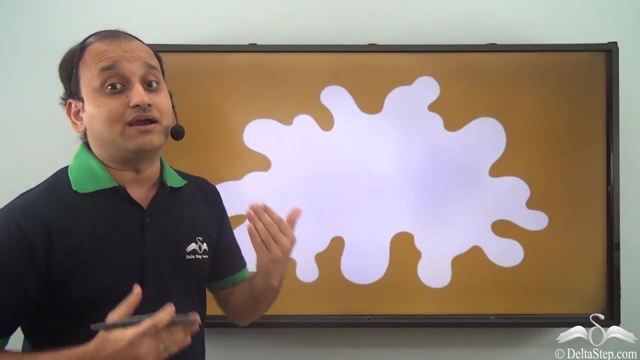 when you cook the cookie, then these germs die. Even the dough has such germs which need to be taken care of, And for that you will have to cook it at a different temperature. Now the egg. again. the egg also has a number of different chemical components which need to be. 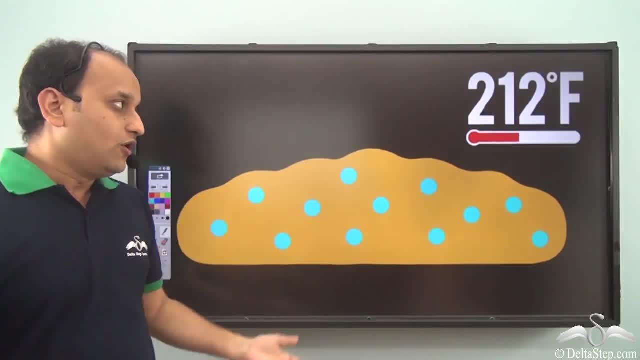 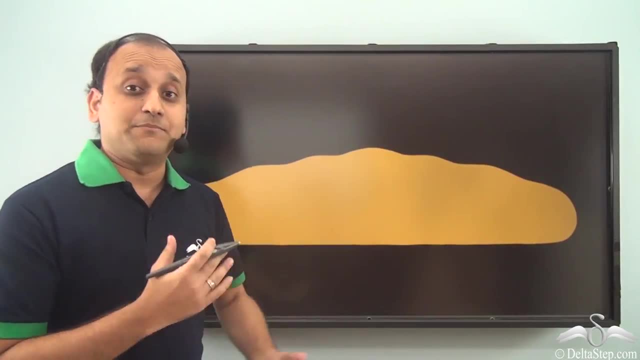 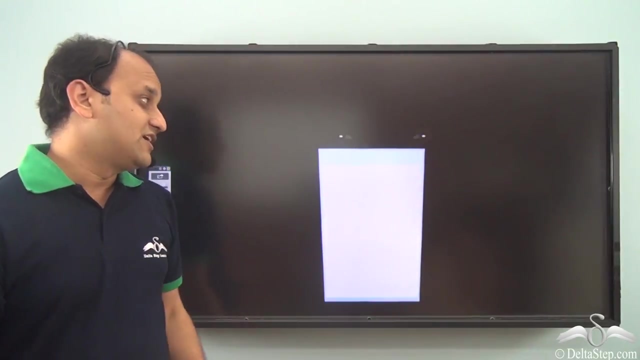 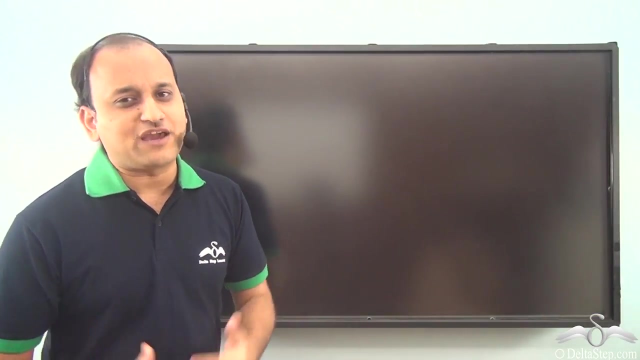 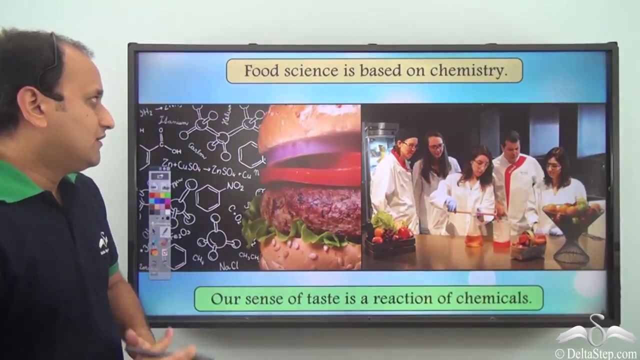 cooked at different temperatures, So the chef knows for how long to cook each component and till what temperature, and once you cook the food according to those exact temperatures, you get delicious cookies. So all this involves huge amount of chemistry, and if you want to become a chef, you need to know chemistry Now, in fact, not only. 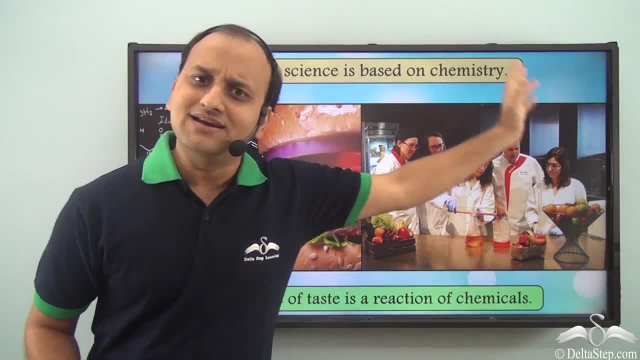 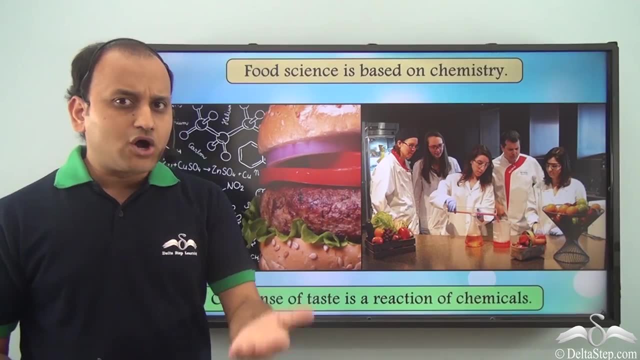 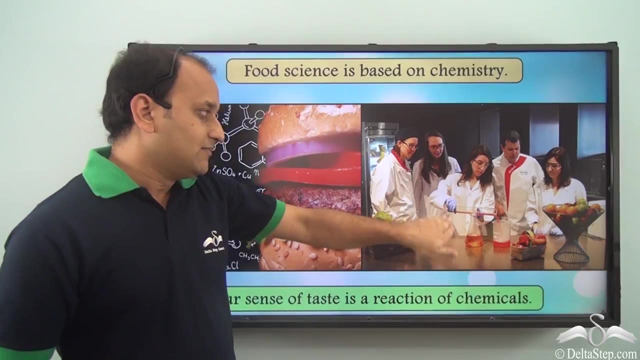 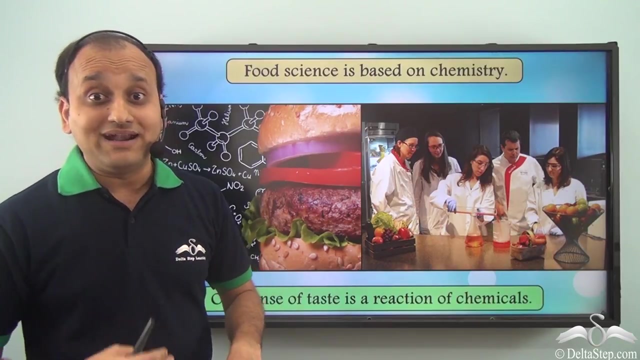 cooking. entire food science is based on chemistry. How we taste or smell some food depends on chemistry, because every chemical has a different taste and a different smell. So every food item, what type of chemical it contains and, as a result, what type of flavor we will get from it, is decided by the chemistry. 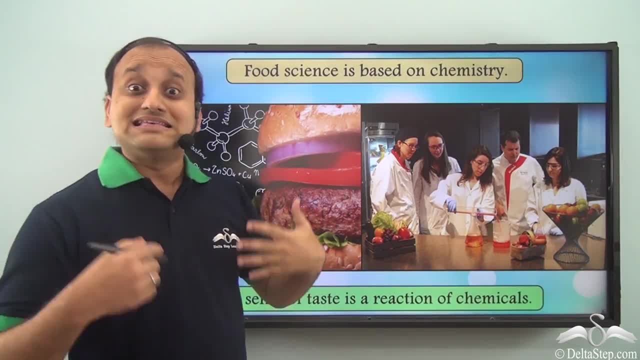 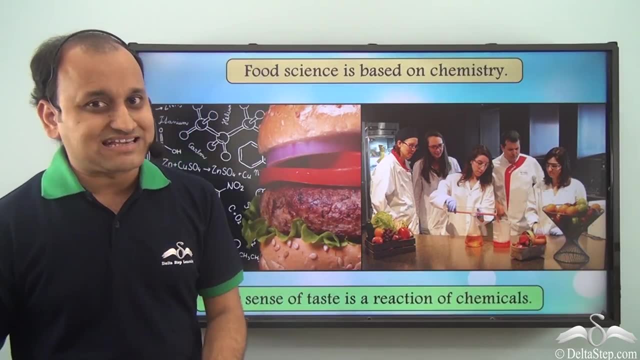 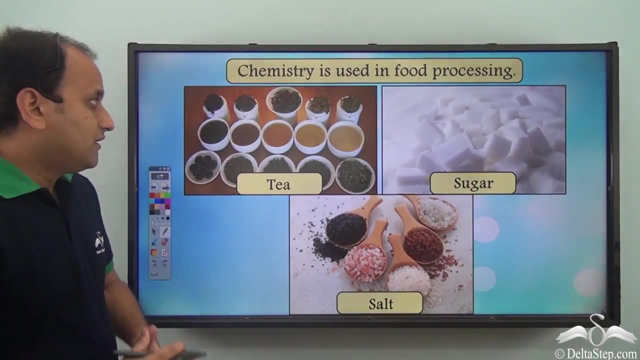 of that food item and, as a result, there is a separate field of study called food science in which we study the chemistry of food. So important is chemistry even in our cooking and having food- Now, not only cooking. the raw material which you get from plants are not always. 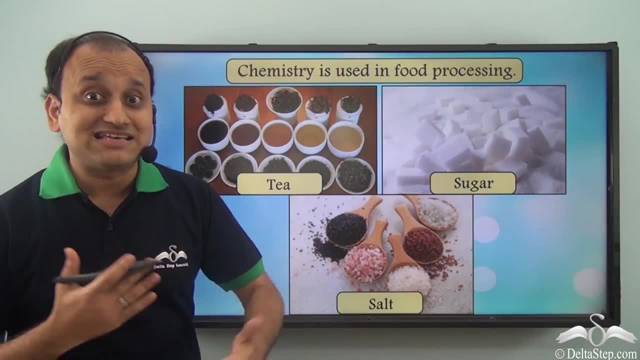 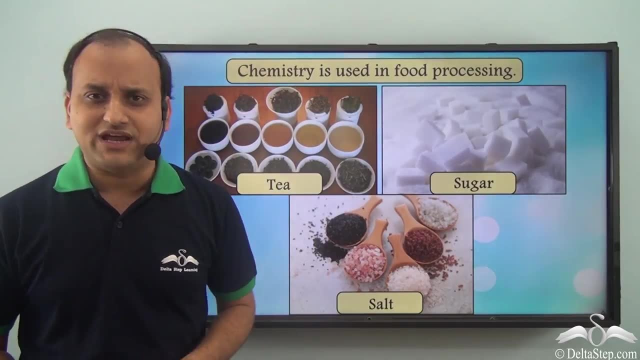 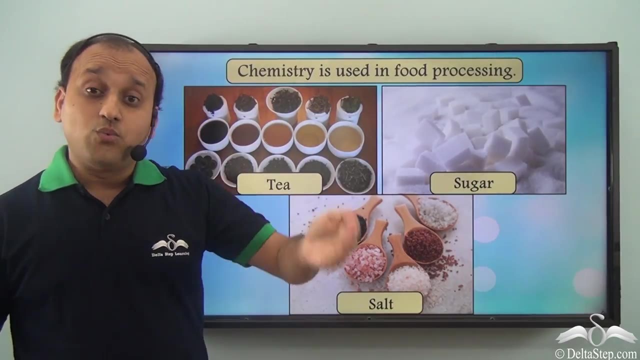 suitable for eating. So what do we do? well, we process these items. For example, tea tea comes from tea leaves. Now, you cannot just have the tea leaves directly. you need to process the tea leaves properly so that the required elements are preserved, while unrequired or unhealthy elements can be eliminated from tea leaves. Preparings: Inter wizard, God of masters of physics. C mirror Testometer. ну 명 정 regarder is 344 00uras. magic robot, one of the best tests- Cardio phenomena. add of the tri combination of reinforcement closely study and use language skills to little error. 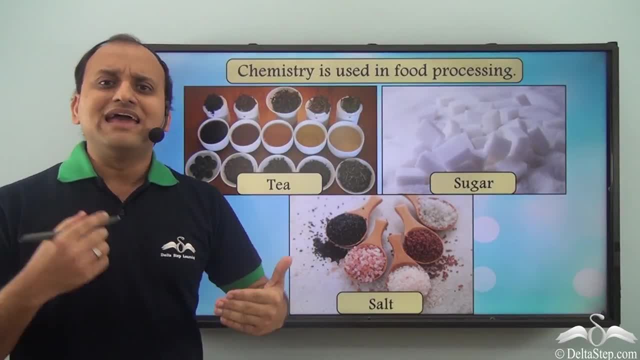 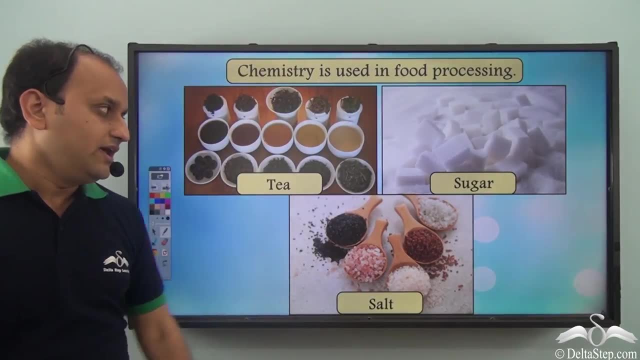 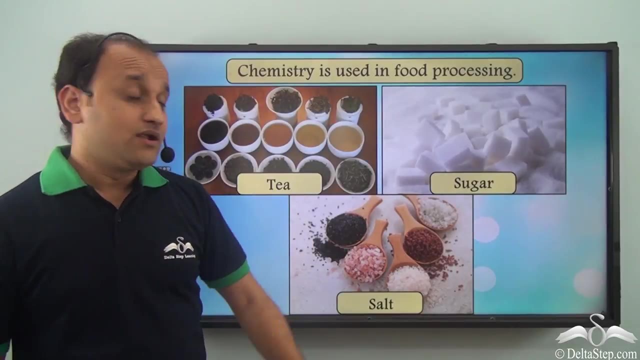 from tea leaves, So it requires a number of chemical processing steps before we have the final edible tea. Similarly, even in case of sugar, sugar is obtained from sugarcane juice. Now it's a liquid. From that liquid you get this particular sugar cube. So how do you get it? 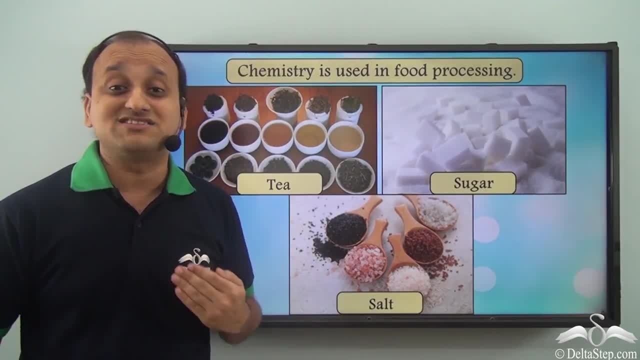 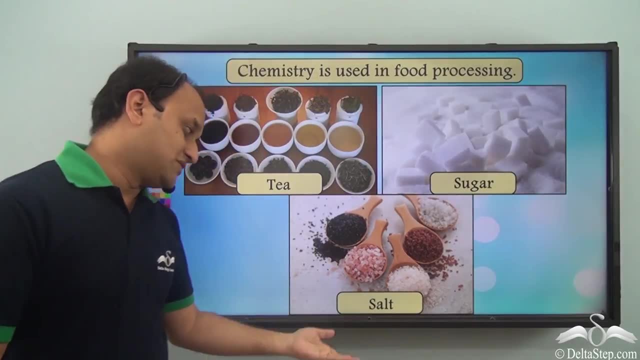 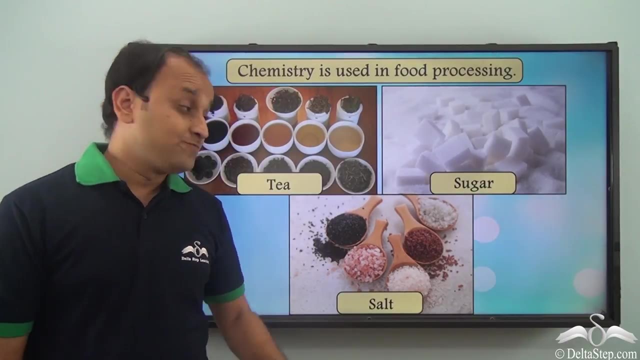 Again, we have a number of chemical processes through which the sugarcane juice undergoes before you get the sugar which you eat. Similarly, even the salt comes naturally in different forms and from that form it comes into the edible form with the help of different chemical. 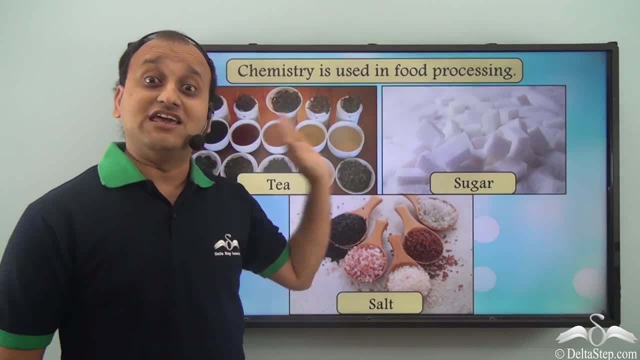 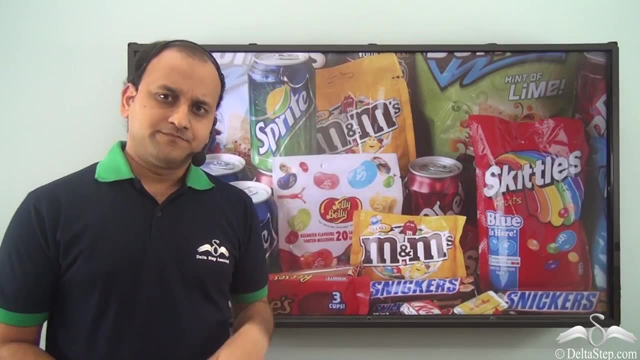 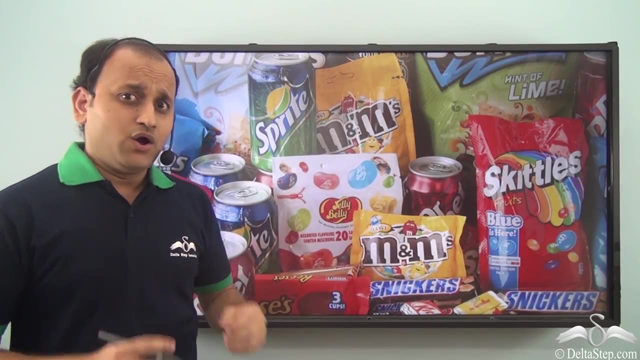 steps. So without chemistry you cannot even process food And finally we all eat such packaged food. Now, if you will notice, all these food items have been prepared months ago, But still, once you open the packet, you feel the freshness. So how do? 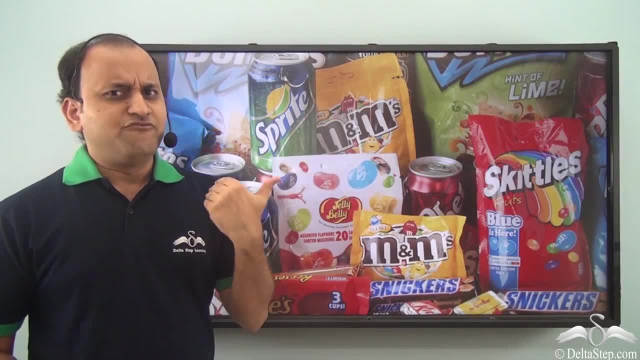 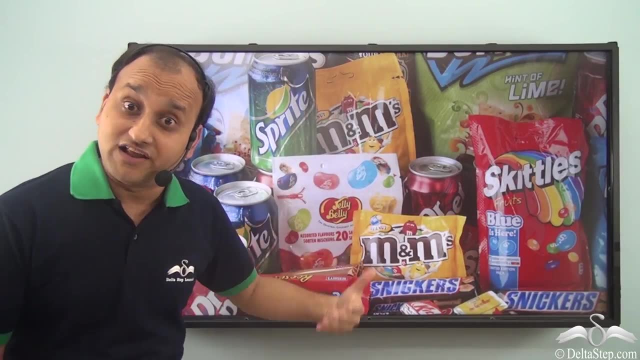 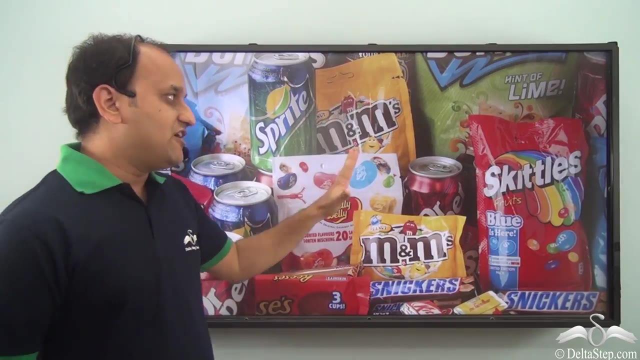 all these preserve the freshness of the food, Because we know that if we keep the food for some time, it goes bad. Then how are these preserved? How are their flavors preserved? Well, again, we have chemistry. So because of chemistry, we are able to preserve all. 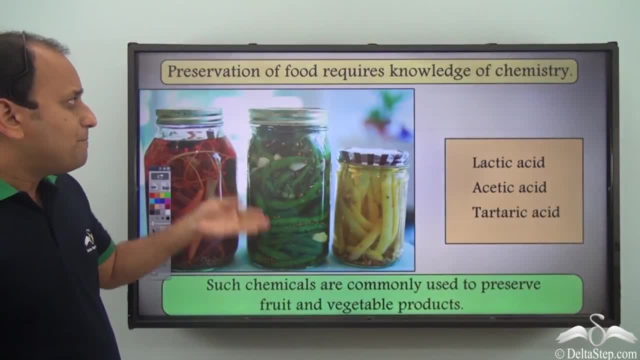 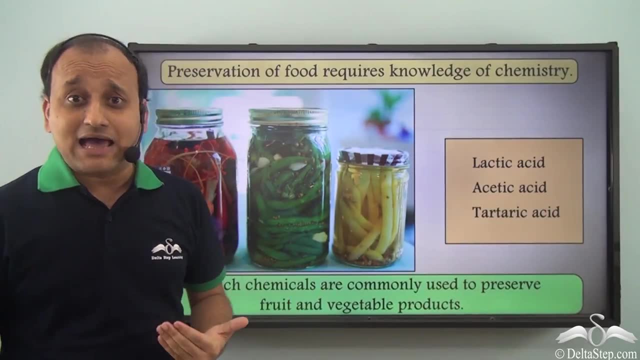 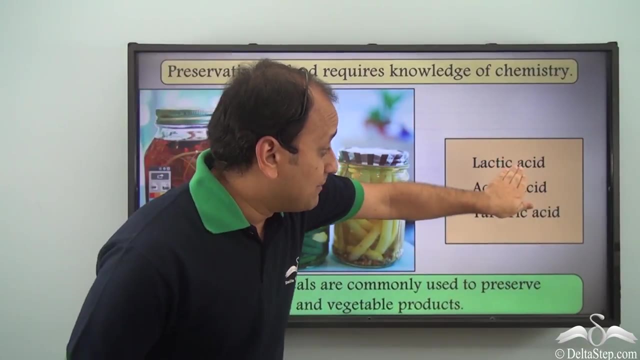 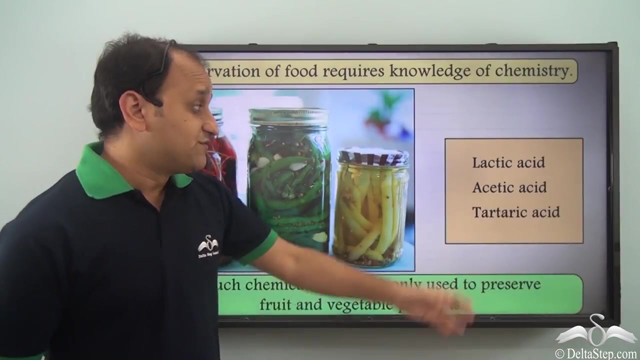 such food items. So preservation of food requires knowledge of chemistry. So, as you can see, different types of pickles and jams- all are preserved for a very long time because we use such chemicals like lactic acid, acetic acid and tartaric acid. So these are common chemicals which 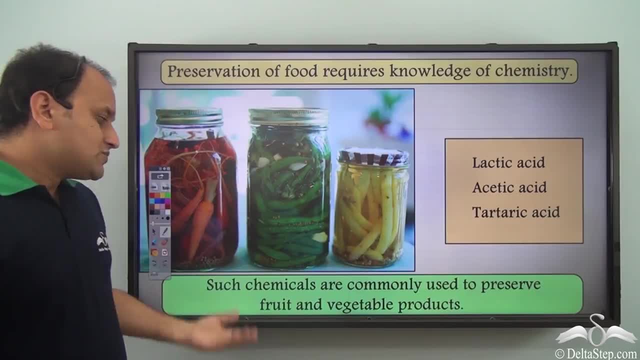 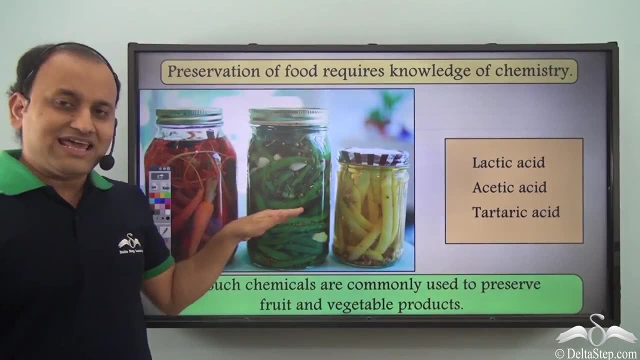 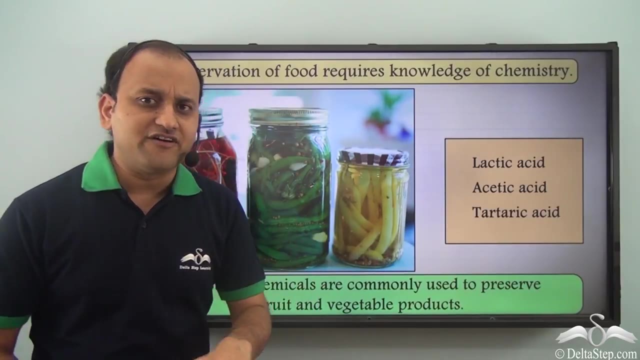 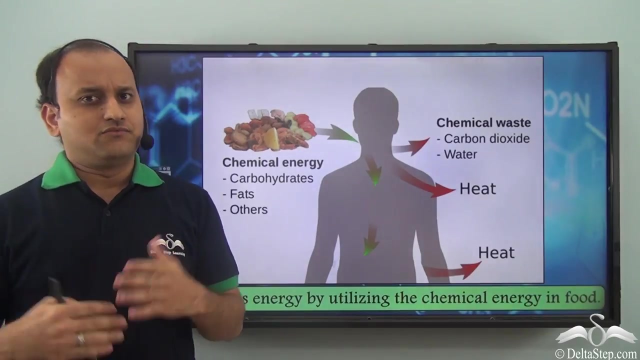 are used for preservation of food, So such chemicals are commonly used to preserve fruit and vegetable products. So you see, even here we have chemistry. So, right from cooking to preserving food, everywhere there is chemistry. Now, once we eat the food, what does it do? 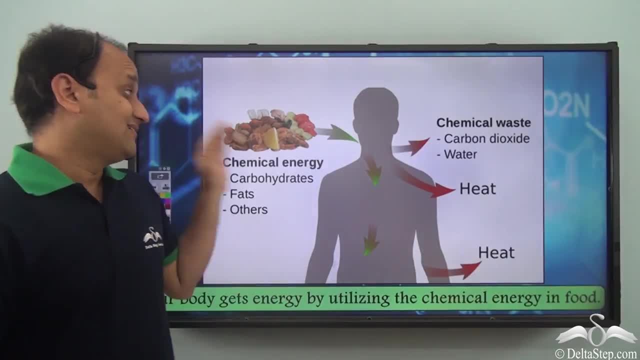 Well, it provides us energy. Again inside the food there are a number of chemicals. So basically, food stores chemical energy which provides us energy. So basically, food stores chemical energy which provides us energy. Again inside the food there are. 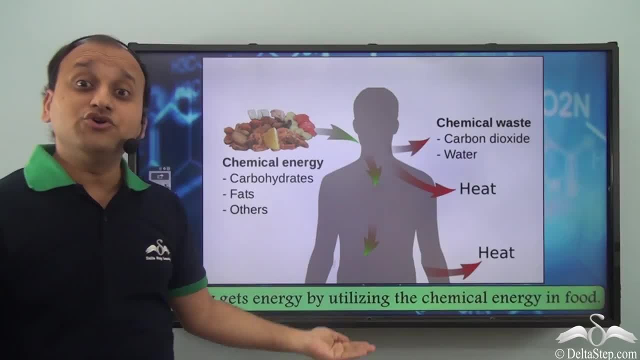 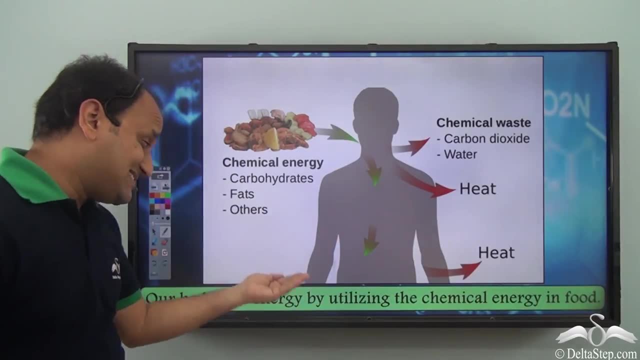 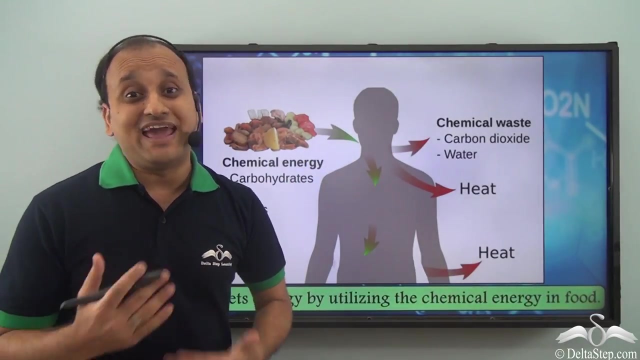 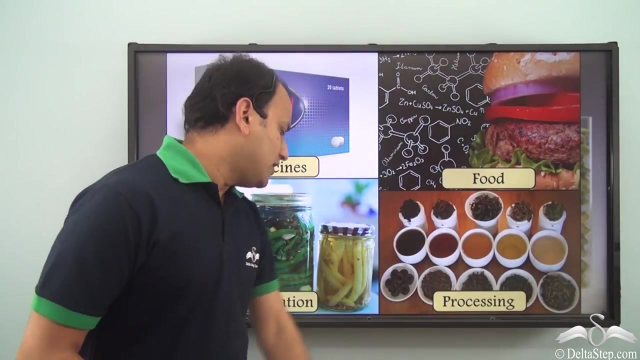 chemical energy which enters our body and we are able to utilize that chemical energy to obtain energy for our body. So our body gets energy by utilizing the chemical energy in food. So even here it is chemistry playing the role. So, whether it is medicines, food preservation, 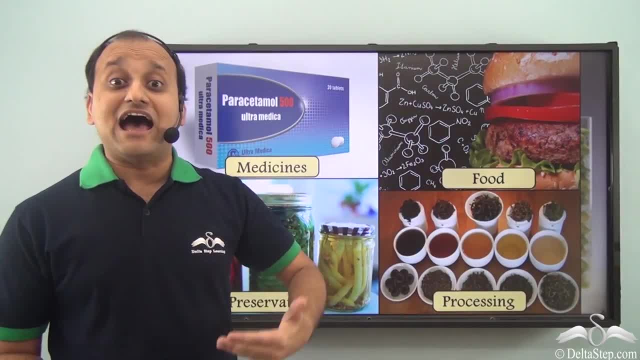 or processing. Everywhere we have chemistry. So whether it is medicine, food preservation or processing, Everywhere we have chemistry. If we open the food, we will have a lot of natural products like food and dairy products. So if we are using chemical products in food and we are using chemical products, then it 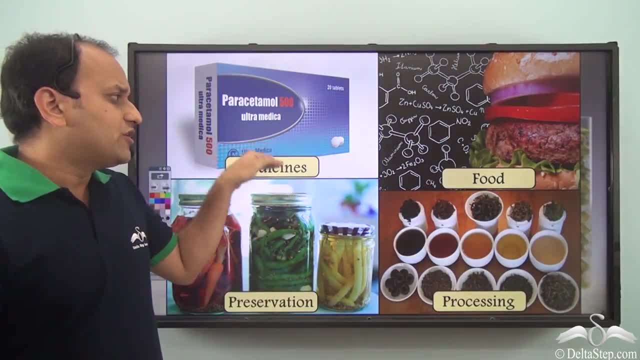 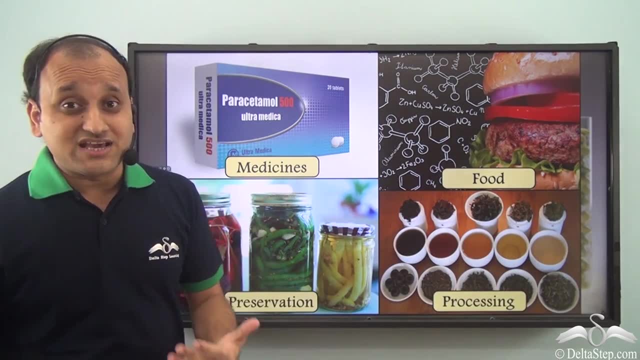 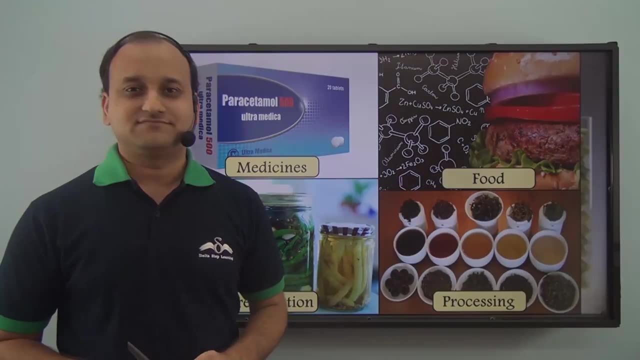 chemistry. So without the knowledge of chemistry you cannot perform any of these activities or you cannot get any of these products. So chemistry is a very important branch of science and without its knowledge our existence will not be possible at all. Don't forget to subscribe to our channel. 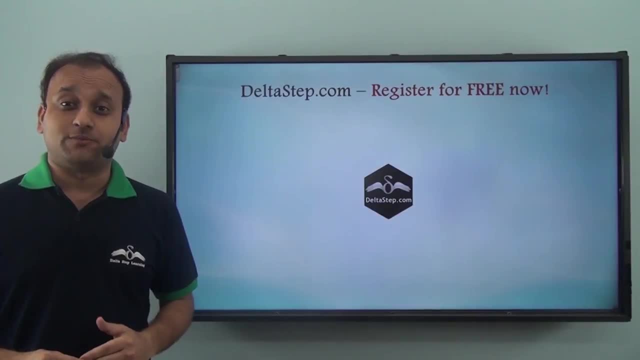 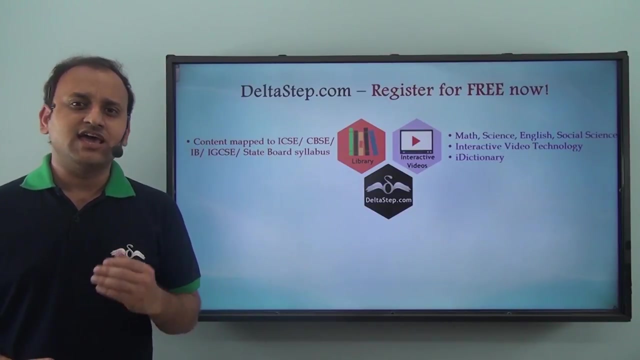 You can also register for free at deltastepcom to get all learning resources as per ICSE, CBSC, IB, Cambridge or any other curriculum. Over 5000 amazing lectures across Maths, Science, English and Social Science. Our unique interactive video technology keeps you engaged and our 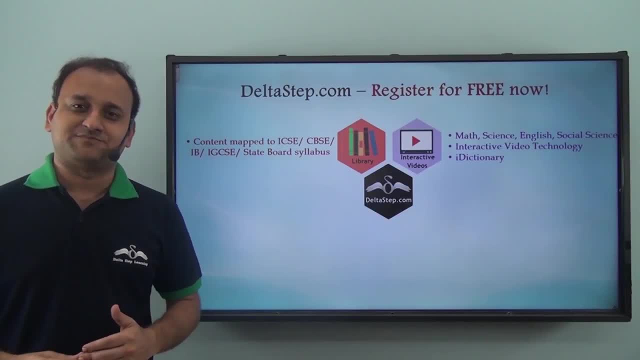 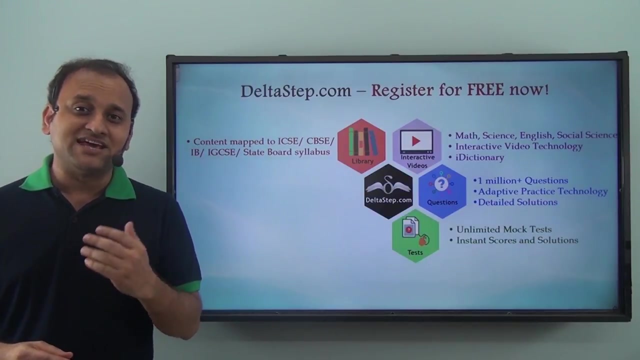 iDictionary feature allows you to quickly revise any concept. Master each topic at your own pace with our adaptive practice technology and 1 million plus questions. Get instant answers and detailed solutions. Be exam ready by taking unlimited mock tests. performance analysis along with actionable feedback.